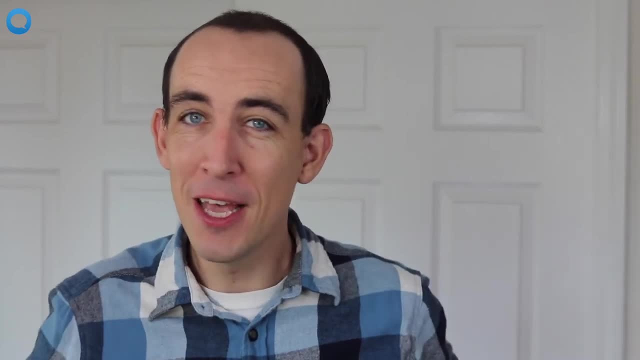 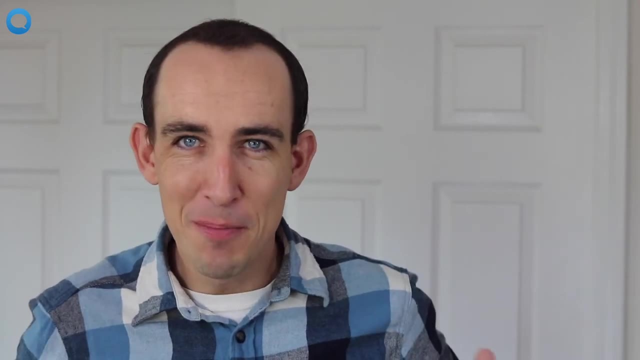 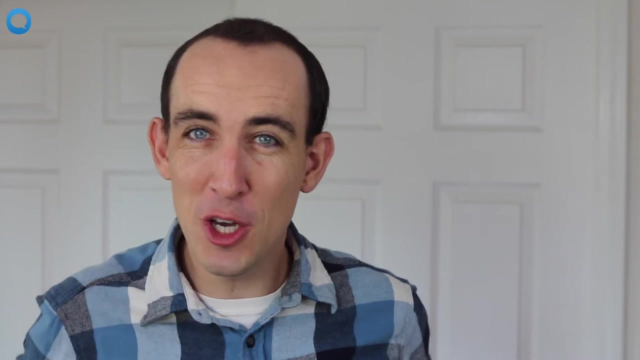 any questions for me that you would like me to answer, just let me know in the comments and I will do my best to answer them in a video for you. Before I start, make sure you download my free book called English Quick Fix, if your goal is. 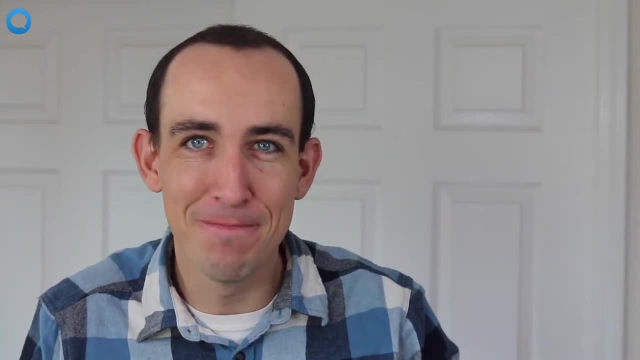 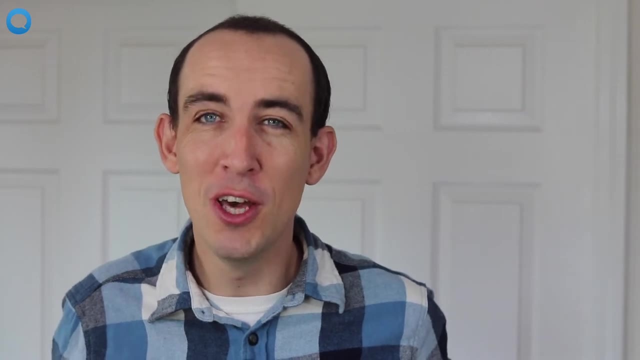 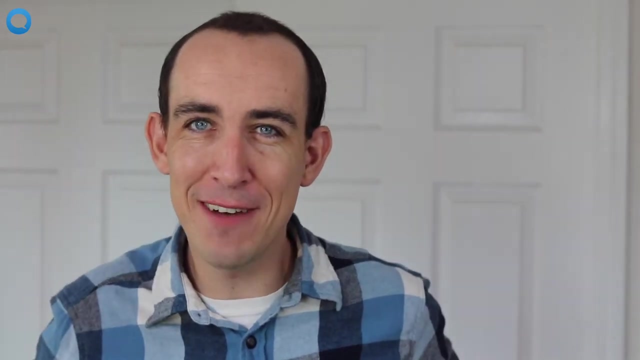 to take your English to the next level, Right? let's have a look at the next question. Let's have a look at the comparatives and superlatives in English, which students so commonly make mistakes with, and it's very simple. So let's have a look at the. 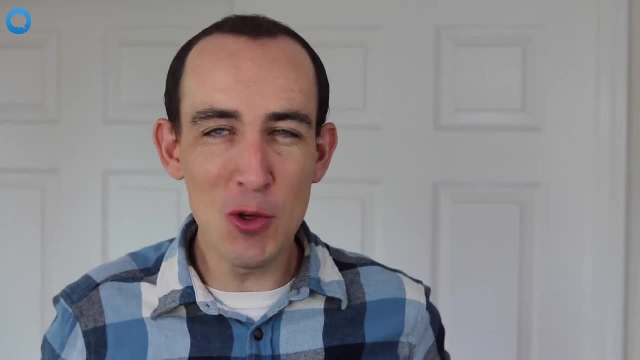 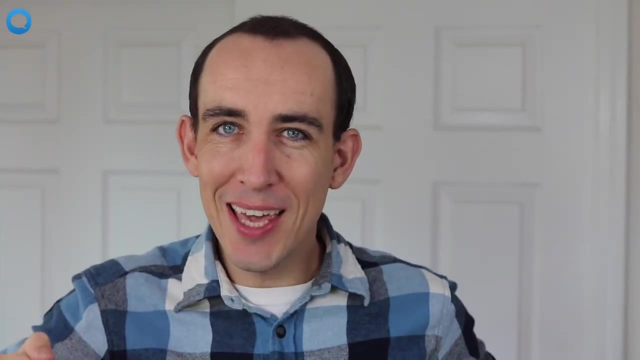 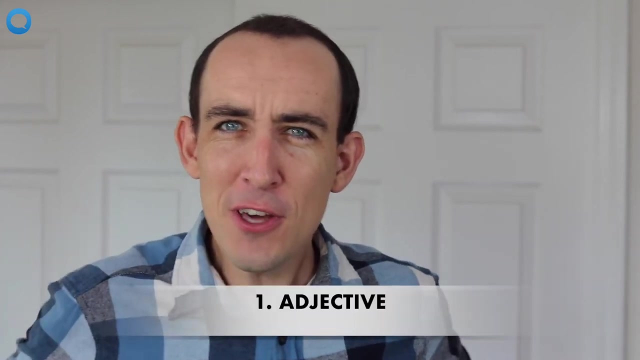 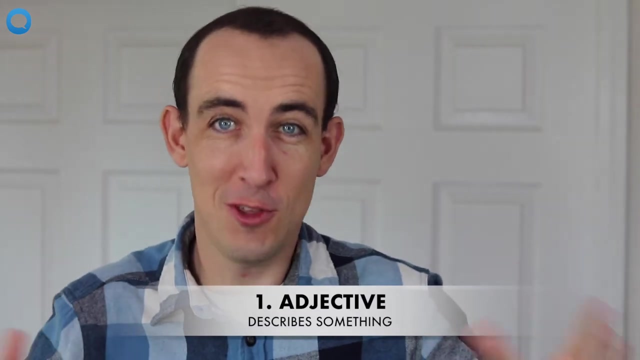 rules and some examples so that you can use it correctly and sound a more advanced speaker of English. So we're going to be looking at an adjective, a comparative and a superlative. So first an adjective. What is an adjective? Well, an adjective simply describes something. 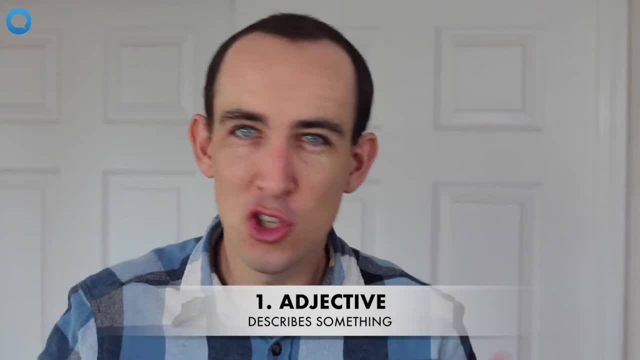 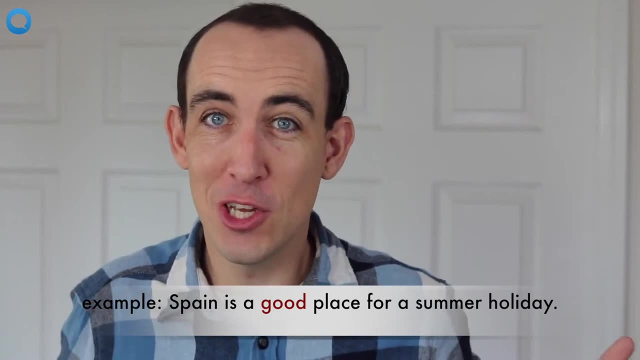 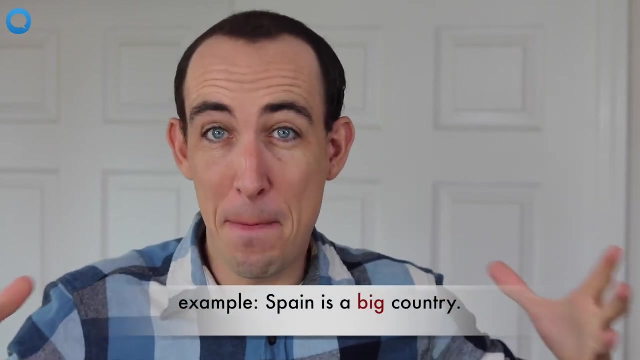 OK, good, red, tall short. For example, Spain is a good place for a summer holiday. The adjective is good, Spain is a good place for a summer holiday, Or Spain is a big country. Spain is a big country. 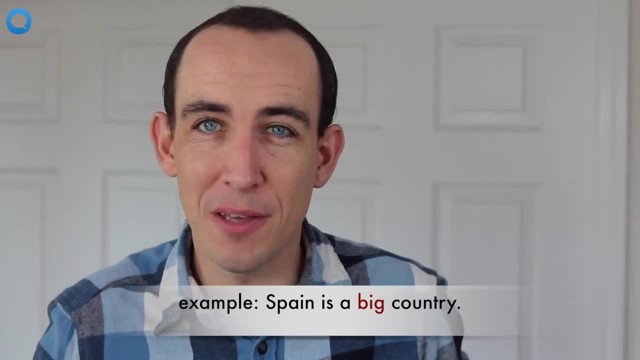 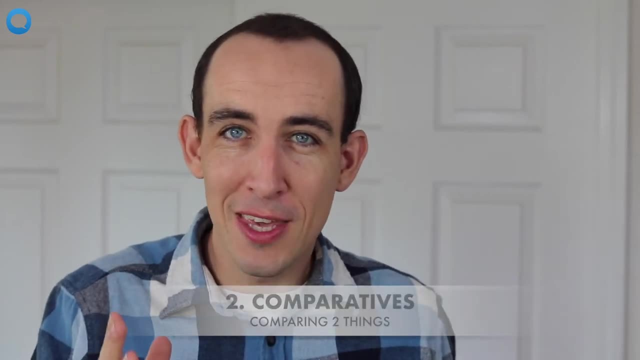 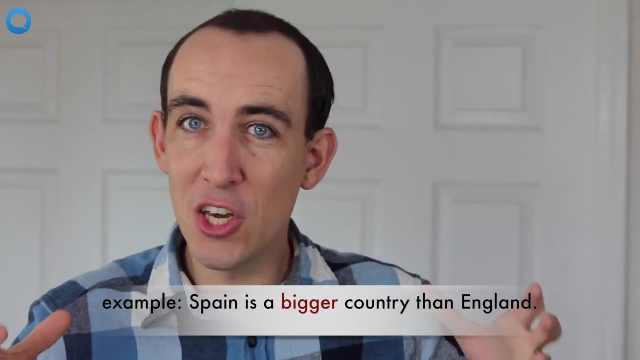 Big is the adjective, Spain is a big country, Simple. So the second thing is comparatives. This is when we're describing two things, Only two things. For example, Spain is a bigger country than England. Spain is a smaller country. 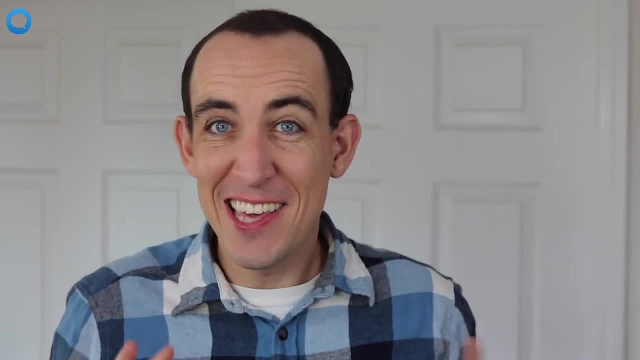 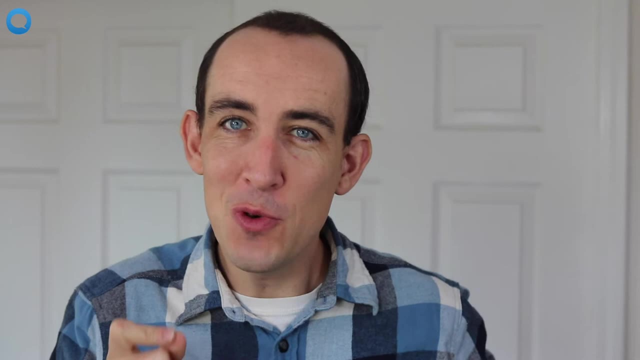 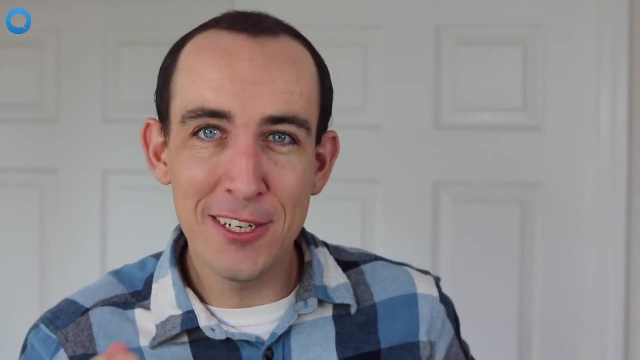 Spain is a bigger country than Russia. To make the comparative is very easy. You simply take the adjective like big, small, tall and you add the schwa sound to the end of that adjective. And if you want more tips on where to use this schwa sound, 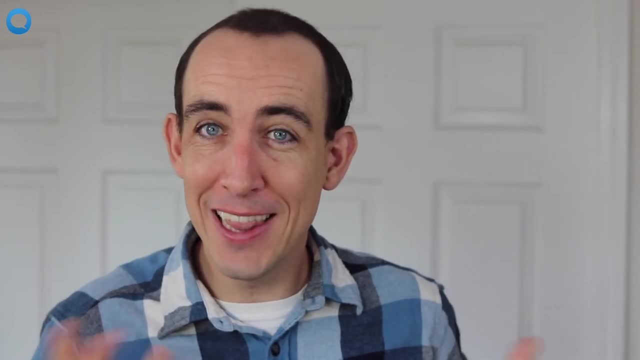 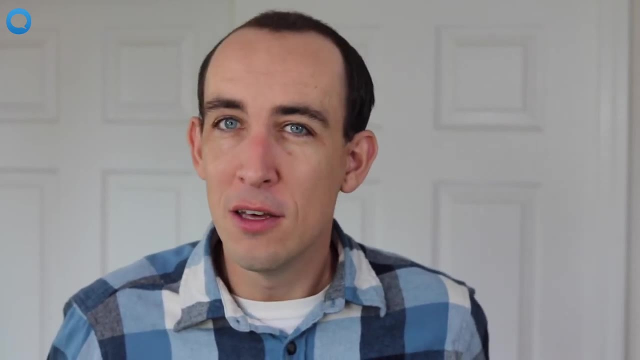 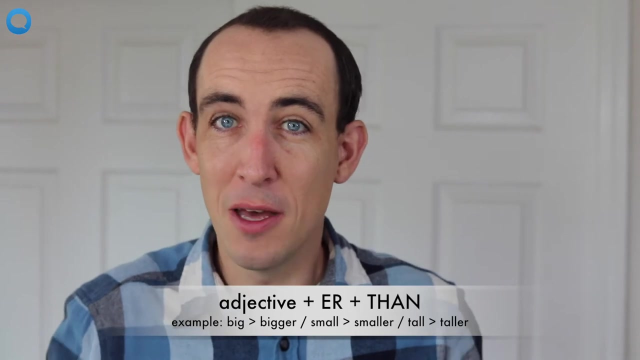 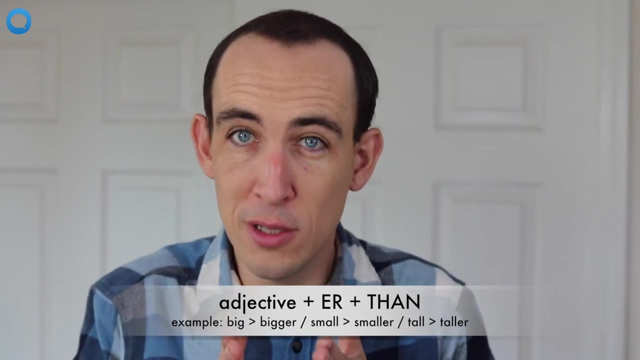 just check out that video and I'll also leave a link in the description. So the schwa sound is All right. So you simply add that to the end of the adjective Big, bigger, Tall, taller, Small, smaller. 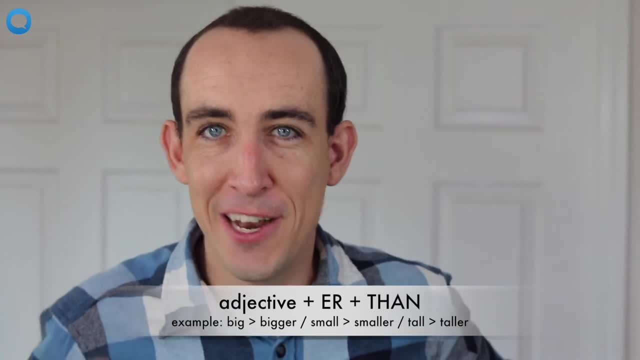 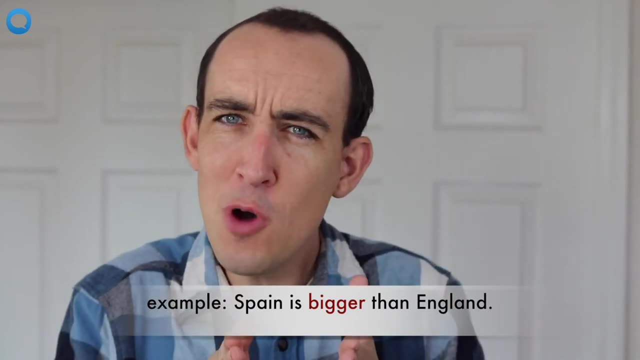 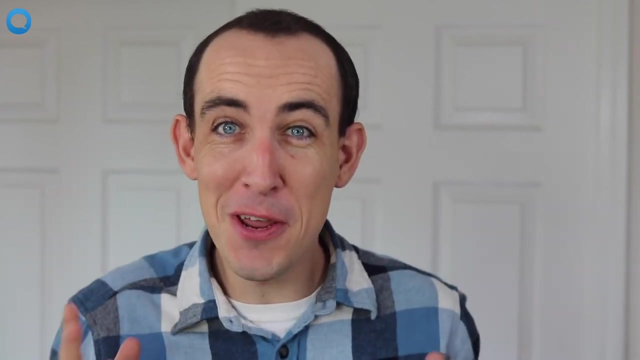 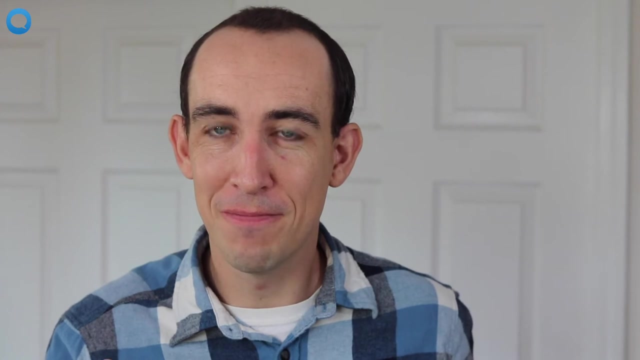 And we follow this with the word THAN. Spain is bigger than England. Spain is smaller than Russia. Now, in English there are always exceptions, And a very common exception with the comparatives and superlatives is for the adjective good, We don't say gooder, which we should. 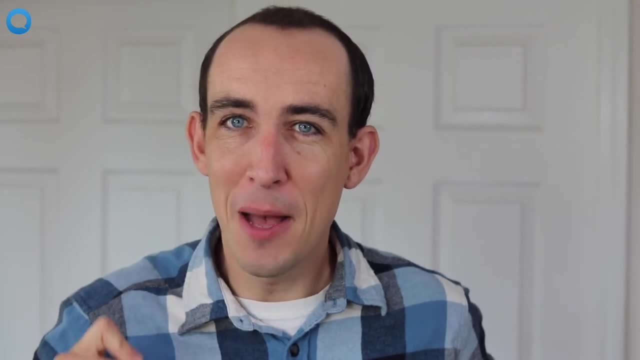 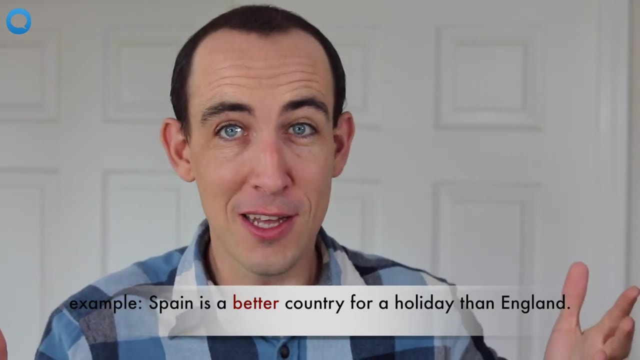 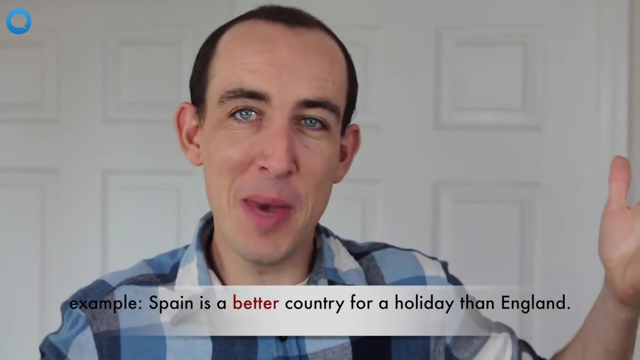 but we use better, Better, Better than Spain is a better country for a summer holiday than England, Because the weather in England is not so good, But the weather in Spain Okay. Third, we're going to look at the superlative. 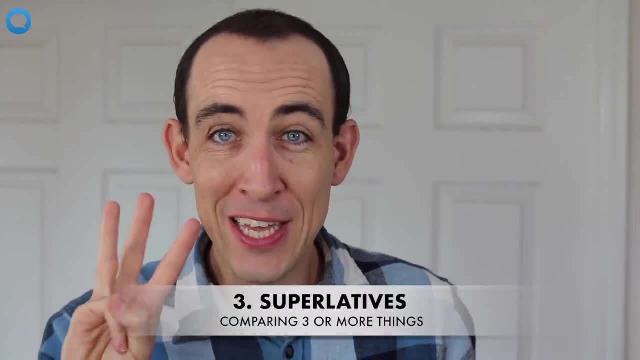 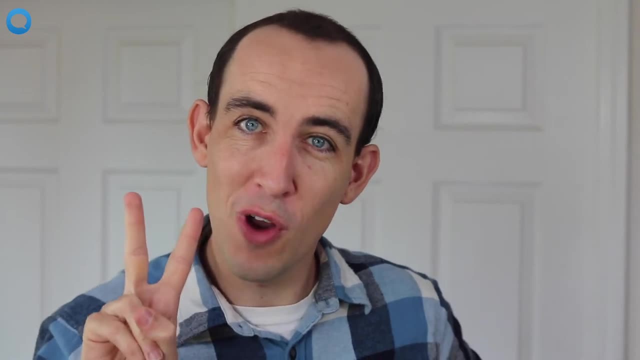 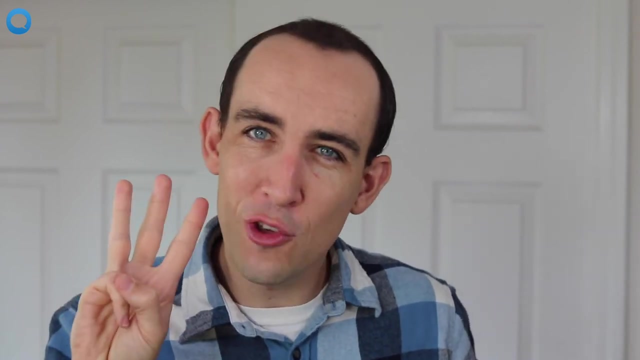 And we use the superlative when we are describing three or more things. So, remember, we use the comparative when we describe two things, Spain is bigger than England, but we use the superlative when we describe three or more things. things To make the superlative, we simply add: 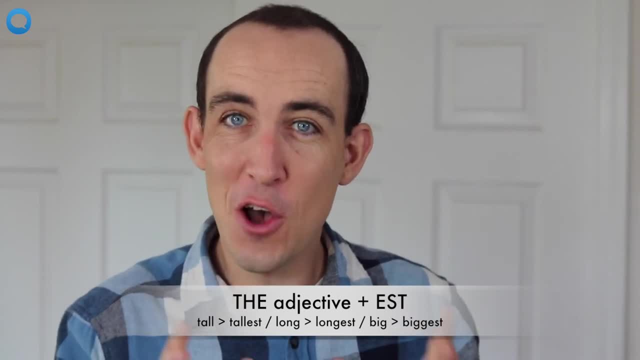 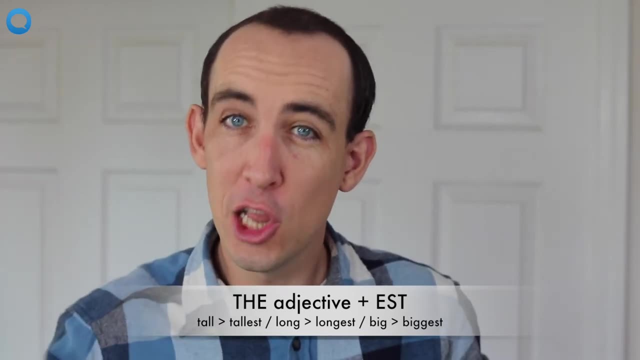 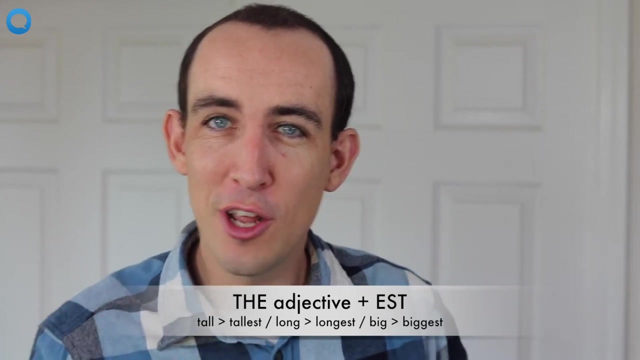 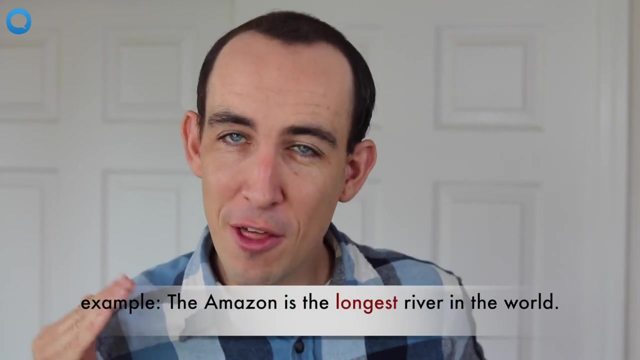 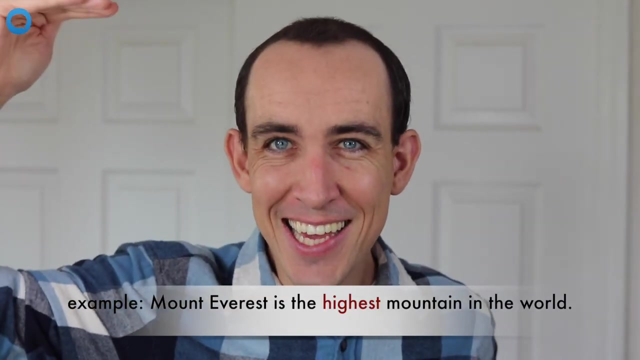 "-ist, "-ist" at the end of the adjective. So tall, tallest, tallest, long, longest, big, biggest, and we always put the word the before the superlative. So, for example, the Amazon is the longest river in the world, Mount Everest is the highest. 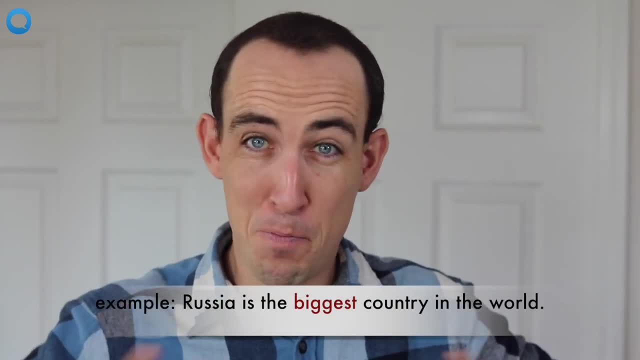 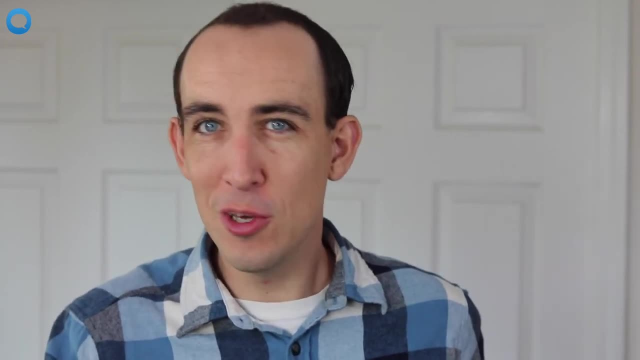 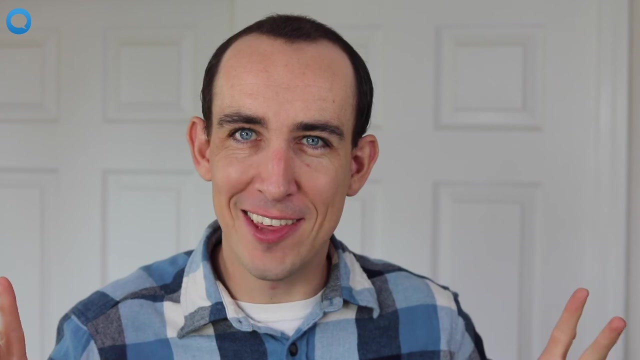 mountain in the world. Russia is the biggest country in the world. We talked about the exception with good. If you want to use good in the superlative, then you use the best, The best. So now I've got a question for you. 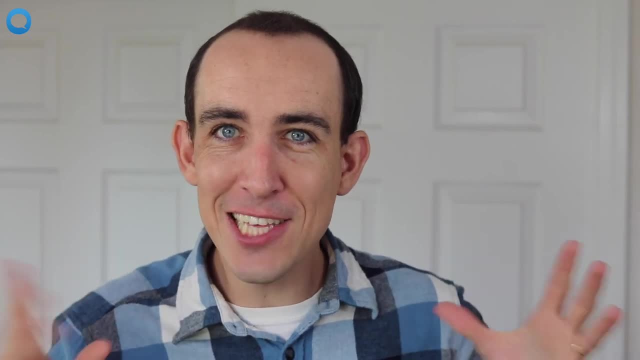 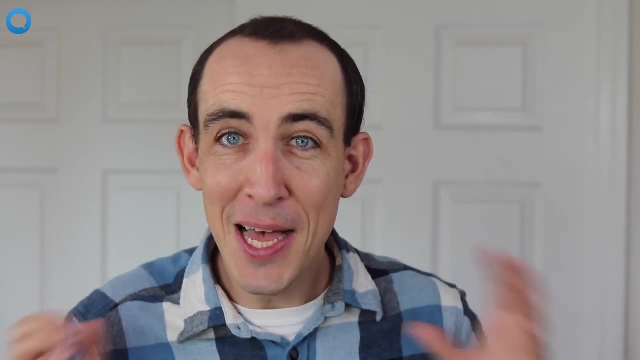 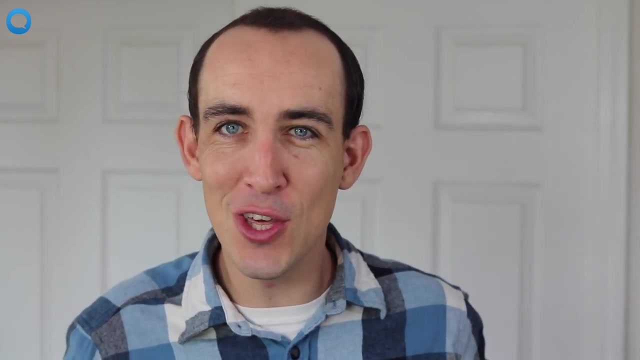 It's almost summer and I want ideas for my summer holiday. In your opinion, which is the best place to go for a summer holiday? Please let me know in the comments. I really want your ideas for my summer holiday this year, So let me know What's the best place for a summer holiday.